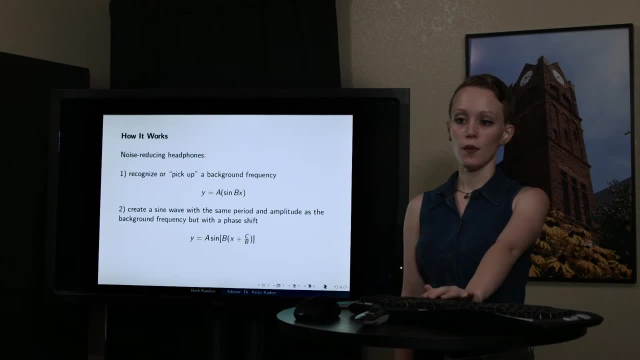 phase shift. So here we have the same equation, but with a phase shift, And then the two notes cancel each other out. It's really hard to see from this how that works, So I'm going to show it graphically. So let's say that we have the note a above middle c, which can be described by sine of. 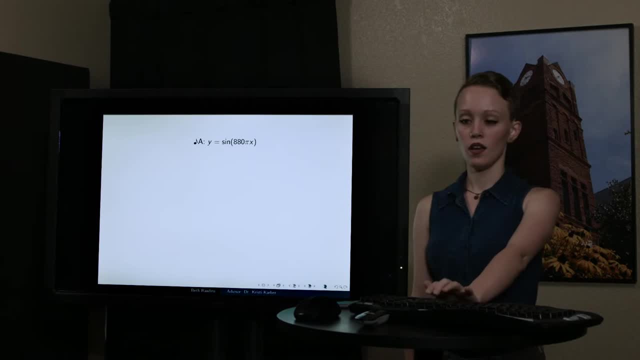 880 pi x. So in this instance our amplitude is 1.. So here's the graph of sine of 880 pi x, And the frequency is going to be 440.. So then we have an a with a phase shift which 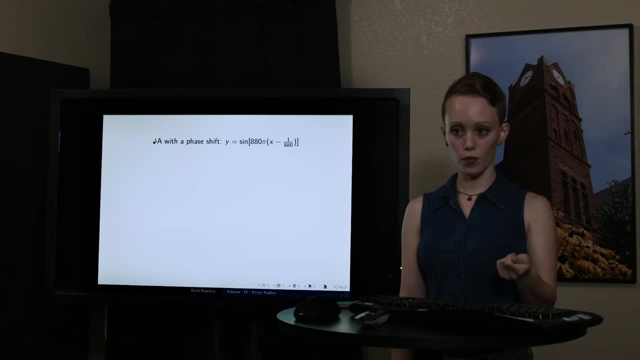 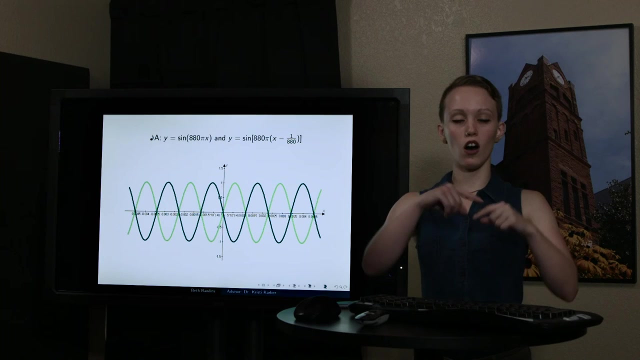 is the signal that the noise reducing headphones would output, And our phase shift is negative: 1 over 880.. And here's the graph of that one. Now notice, when we show them on the same axis, that they oscillate opposite each other, And so in this way you can kind of see how they would cancel each other out. 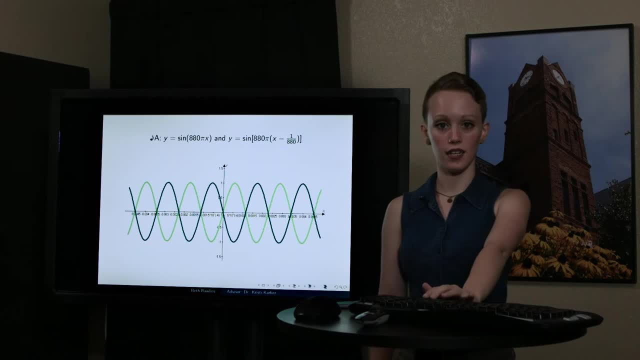 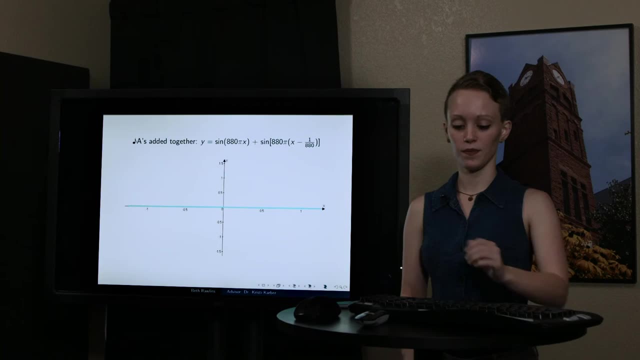 Now we could use analytically a trigonometry identity to show how, when you add these two equations together, you just get the line of y equals 0, which is basically the line of silence. Now, one cool thing that I found that you can kind of play around with to see the relationship. 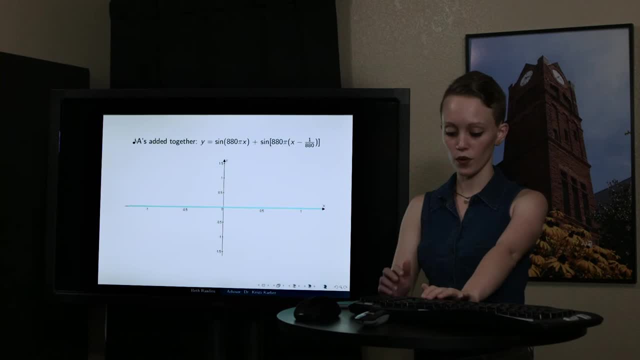 between sine waves and sound waves. is there's an app where you can so say we wanted to play? let me go back here. Say you wanted to play the note sine of 880 pi x. I'll leave the graph on So you can input. you can calculate the frequency which we said was 1 over the. 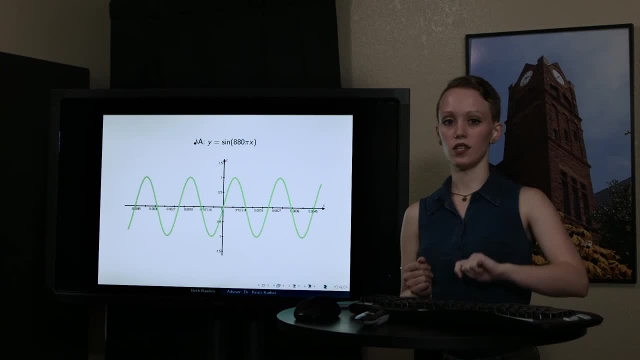 period, And since the period is 2 pi over b, the frequency is going to be b over 2 pi. So in this case our b is 880. pi over 2 pi would be 440.. The app is called NCH Tone Generator. 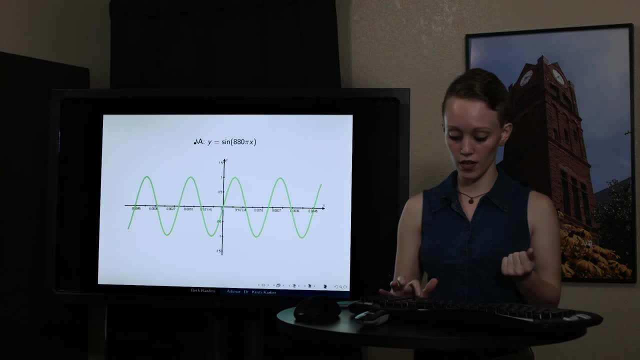 It's totally free And it'll give you a sine frequency and you can edit it. And let's say I wanted to input 440 hertz. Then I can play the note and hear what this equation actually sounds like as a sound wave And you can play around with it with different equations and kind of see. 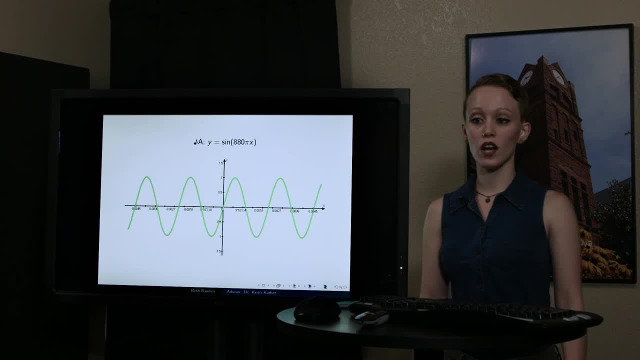 how that works. It's a pretty cool application And there's lots of fields that use this information, such as sound engineering. Musicians use this information and, yeah, that's pretty cool. I think that's all.